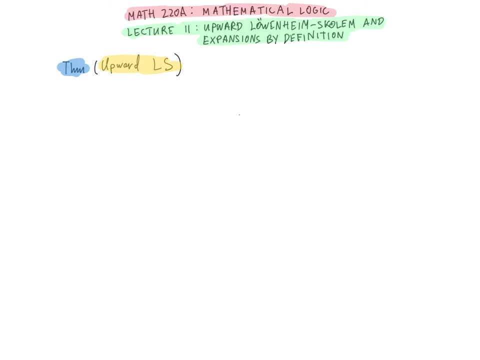 We already saw the downwards Leuvenheim-Scholem theorem, which allows us to find elementary substructures of smaller size in particular, And now we are interested in finding elementary extensions of arbitrary larger sizes of a given structure, M. So, towards this purpose, let M be an infinite L-structure. 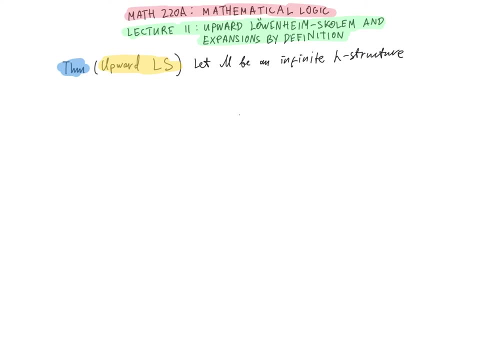 for some language L, and let kappa be a cardinal, such that kappa is greater or equal than the cardinality of M plus the cardinality of the language L, Then there exists an elementary extension of M which is of cardinality. kappa Proof. 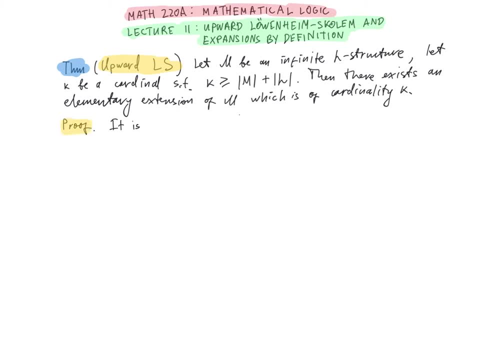 First note that it is enough to construct an elementary extension n of M of cardinality greater or equal than kappa, and then to apply the downwards Leuvenheim-Scholem theorem to a subset A of n of cardinality kappa, containing the base set of the structure M. 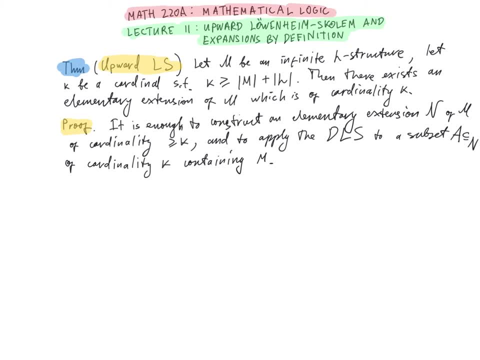 which would give us precisely an elementary extension of M of cardinality kappa. We are using here the following observation: that if we have M an elementary substructure of N, and we also have that M is a substructure of N0, which in turn is an elementary substructure of N. 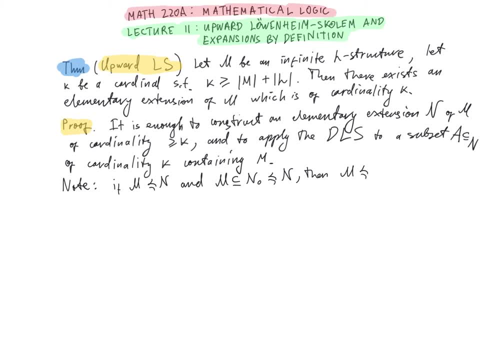 then also M is an elementary substructure of N0.. This is immediate from the Tarski-Watt test. Indeed, assume that phi of x0, A bar is a formula and A bar is a tuple of parameters from M, such that 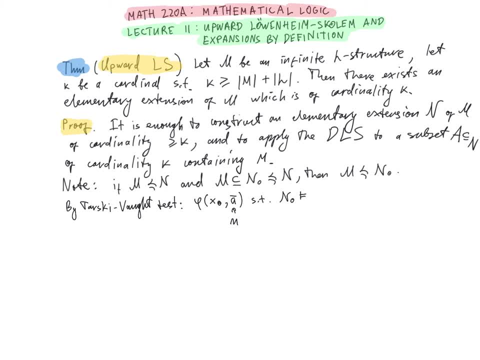 N0 satisfies phi of B0 A bar for some element B0 in N0.. But of course N0 is in particular a subset of N and we also know that M is an elementary substructure of N. so there must exist. 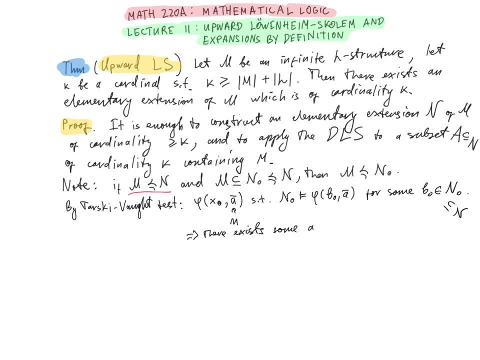 some a, 0 in M, such that we have that N satisfies phi of A0 A bar. but of course all of the elements A0 and the elements of the tuple A bar are in particular in N0, and N0 is an elementary substructure of N. 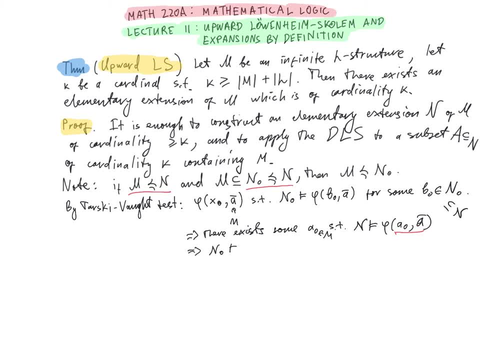 hence we have that N0 satisfies phi of A0, A bar, and A0 is in M. so by Tarski-Watt test, since phi was arbitrary, this implies that M is an elementary substructure of N0. Hence we have reduced the problem. 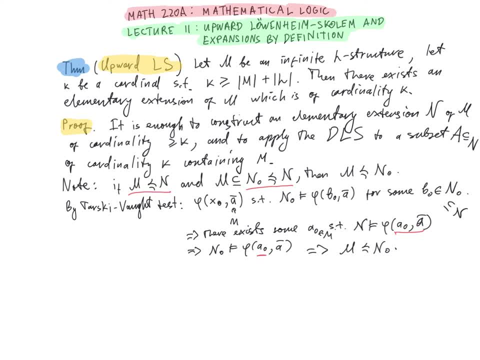 to finding an elementary extension of M of cardinality, at least kappa. So now, for any i in kappa, let c i be a new constant symbol, and we consider the language L tilde, which would take to be the language L m, together with the union. 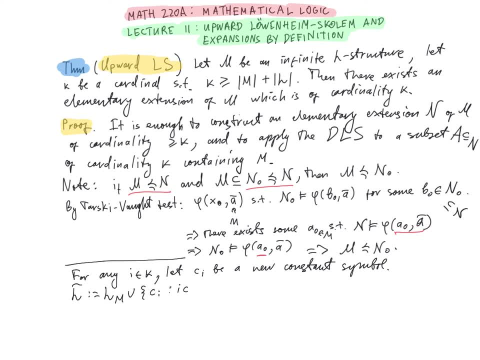 of all these new constant symbols, c? i for i in kappa, and we consider the L tilde theory, T tilde, which we take to be the complete diagram of M, together with the sentences of the form. the negation c i equals c j for all. i less than j, less than kappa. 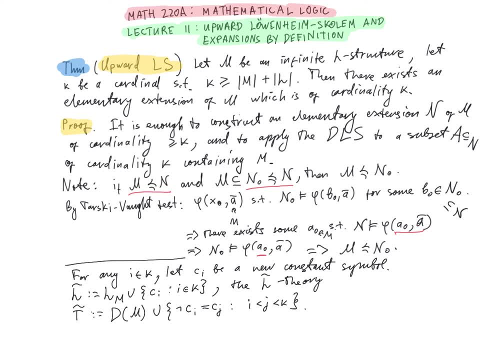 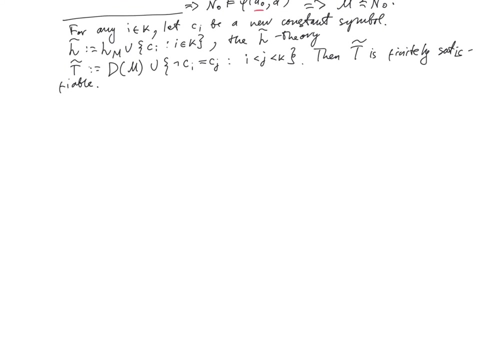 So it's a theory of cardinality kappa. Then we claim that T tilde is finitely satisfiable, meaning that every finite subset of T tilde has a model. Indeed, if T tilde zero is a finite subset of T tilde, 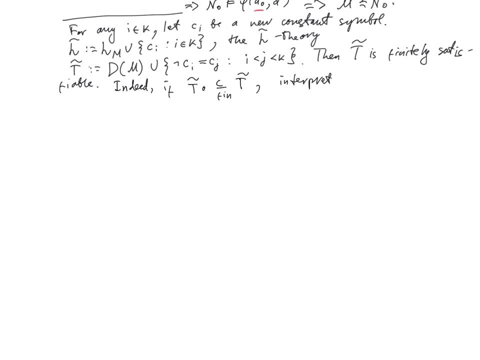 we can interpret the finitely many constant symbols, let's say c i one through c i n, occurring in T, tilde zero, by arbitrary set of distinct elements of M, which is possible to do because we're assuming that the structure M is infinite. 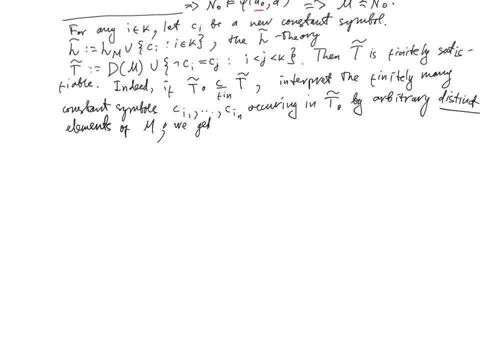 hence we get an expansion of M star, the structure consisting of M with all of its elements named by the constants in the diagram, in the complete diagram language, which is a model of T tilde zero. Hence, by compactness, we get: 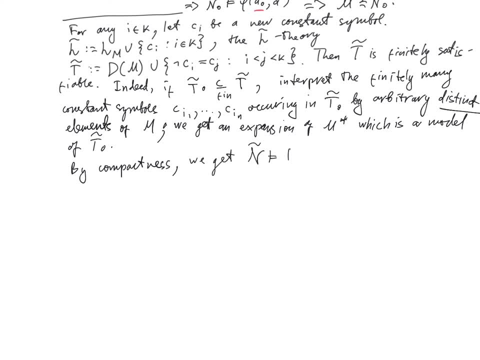 N tilde, a model of the whole theory T tilde, whose L-reduct N is an elementary extension of M, because, in particular, N tilde is a model of the complete diagram of M and, moreover, we have that the cardinality of N tilde. 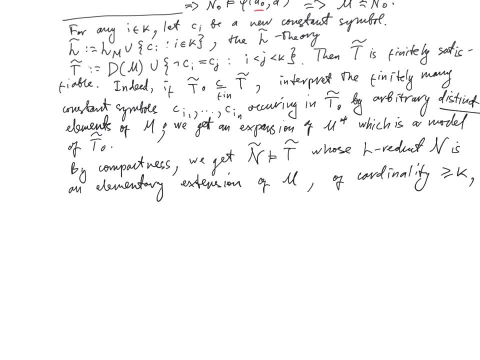 is at least kappa, since it contains the elements c, i. the interpretations of the constants c, i in N, tilde for all i in kappa and the interpretations of these constants have to be pairwise distinct, because this is explicitly stated by the axioms. 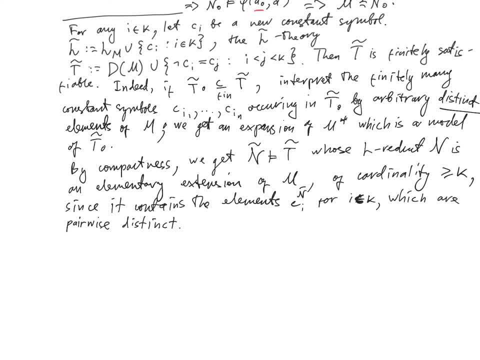 contained in T tilde and N tilde is a model of T? tilde, So this gives us a model of size, at least kappa, and hence, by the earlier discussion we can find a model of size, an elementary extension of M, of size, exactly kappa. 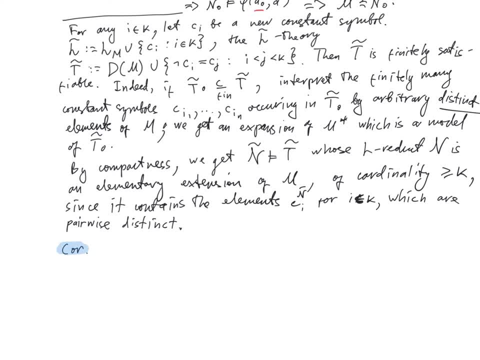 Combining the downwards Leuvenheim-Skolian theorem and the upwards Leuvenheim-Skolian theorem, we have the following corollary: Let T be a theory admitting an infinite model. then T has a model of cardinality kappa. 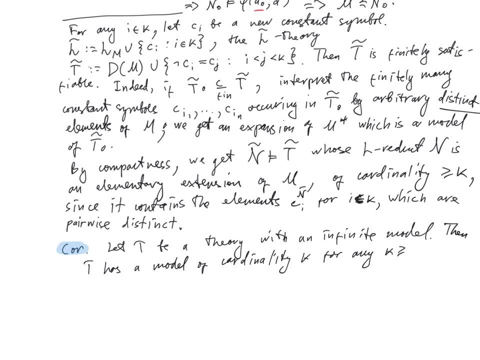 for any kappa greater or equal than the cardinality of the language L. So this tells us that for theories admitting infinite models, the theory absolutely cannot see the cardinality of the model contrasted with the situation for finite structures. So recall that if M is finite, 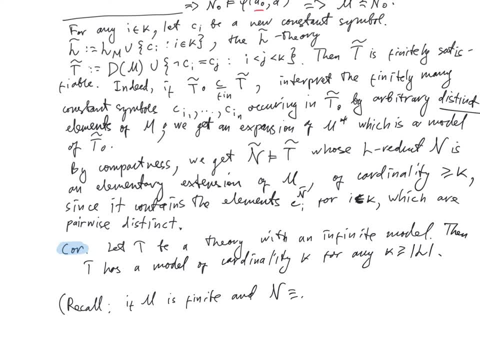 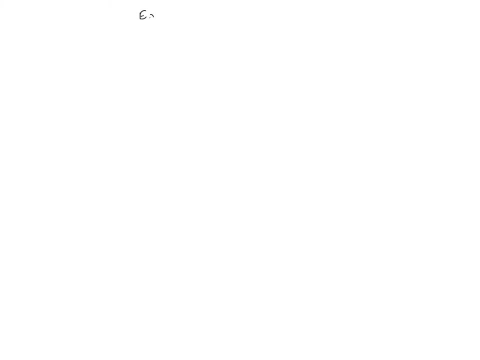 and N is elementarily equivalent to M, then in fact N is isomorphic to M, so in particular it has the same size. Next topic we discuss is expansions by definition. When studying a class of structures in a given language, it might often be useful. 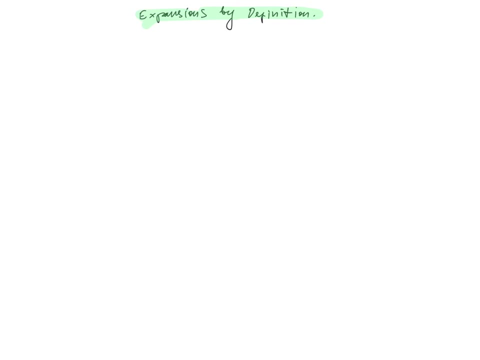 to enrich the language by symbols for definable relations, functions or constants. So here we will describe how this may be done formally without changing the expressibility of the language. We introduce some notation. We will write: exists with an exclamation sign: x, psi. 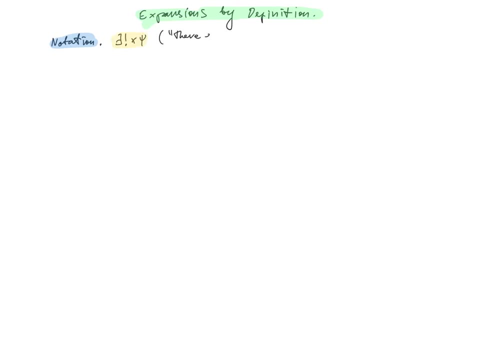 read: as there exists a unique x, such that psi as an abbreviation for the formula exists x, psi and for all x', psi with x'. substituting x implies x is equal to x', With x' a variable distinct from x. Now we have the following definition: 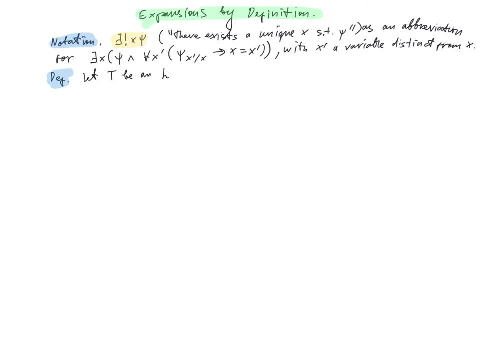 Let T be an L-theory and let L' be some language containing L. Assume that there are the following: for any anery relation symbol R in L' which is not in L: an L-formula phi R of x1 through xn. Next for any. 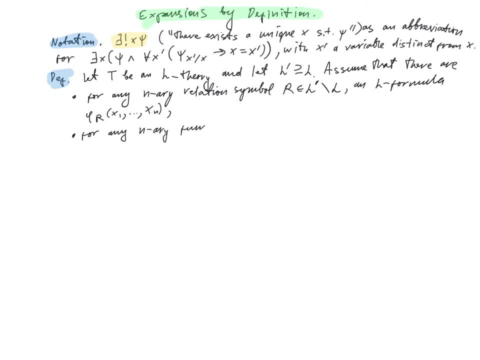 anery function symbol f in L' but not in L, we have an L-formula, phi f of x0, x1 through xn, such that the theory T implies that for all x1 through xn there exists a unique x0, such that phi. and finally, 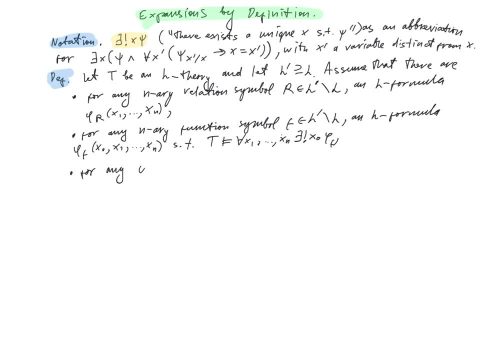 for any constant symbol c in L' but not in L', an L-formula phi c with a single free variable x0, such that T implies that there exists a unique x0, such that phi c. under these assumptions, we have that then the L'. 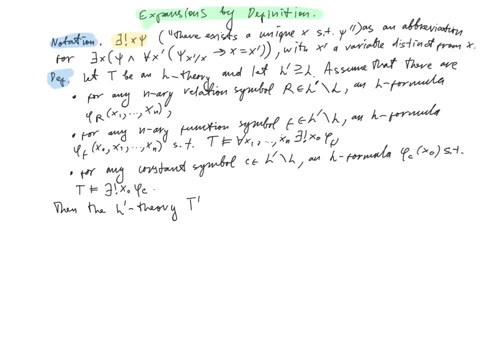 theory T' given by T, together with the following axioms. so first an axiom for all: x1 through xn. phi R of x1 through xn is equivalent to R x1 through xn for any relation. symbol R in L' but not in L' so 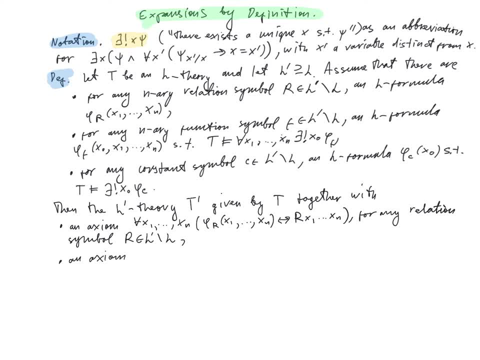 we have an axiom for all: x1 through xn, phi F of F, of x1 through xn, x1 through xn, for any function of x1 through xn. x1 through xn for any function of x1 through xn. for any function of x2 through xn. 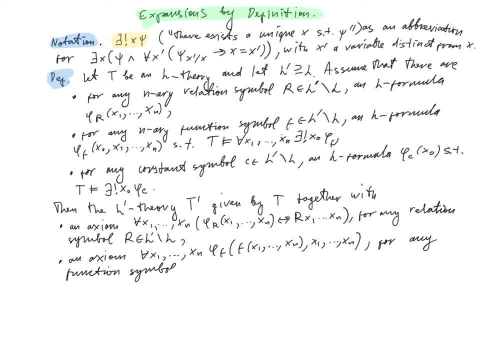 for any function of x3, for any function symbol F in L' but not in L' and also an axiom for xn phi C of C, for any constant symbol C in L prime but not in L. So theory T prime given by T and all these axioms is called 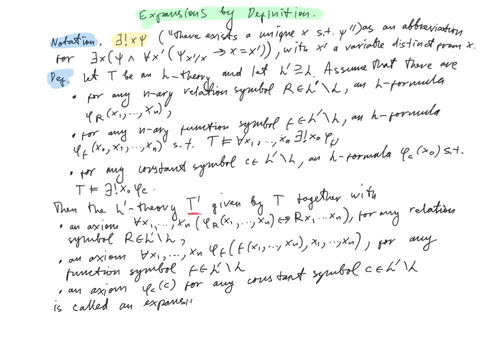 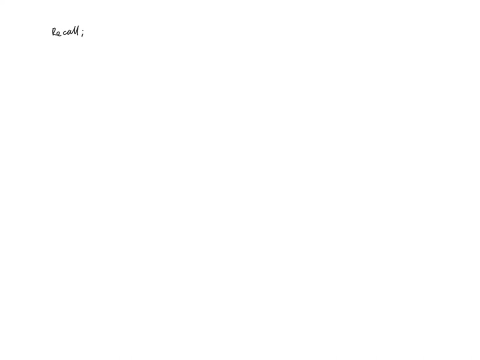 an expansion by definition of T. Recall that two formulas, phi1 of x1 through xn and phi2 of x1 through xn, are called equivalent in the theory T. If we have that, T implies for all x1 through xn phi1 is equivalent to phi2.. 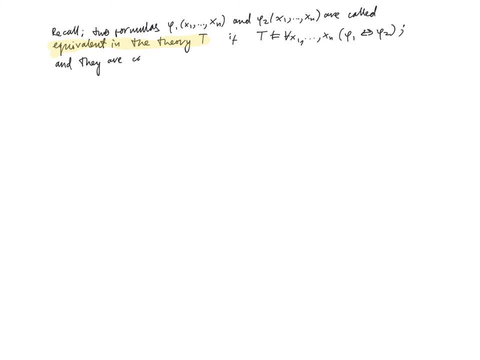 And they are called logically equivalent. If they are equivalent to phi2, they are called logically equivalent. In the empty theory We have the following lemma: Any formula is logically equivalent to a formula with all terms of height less or equal than 1.. 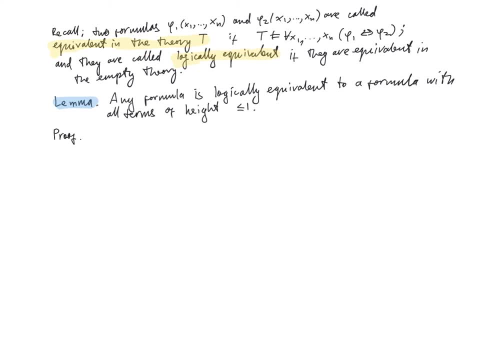 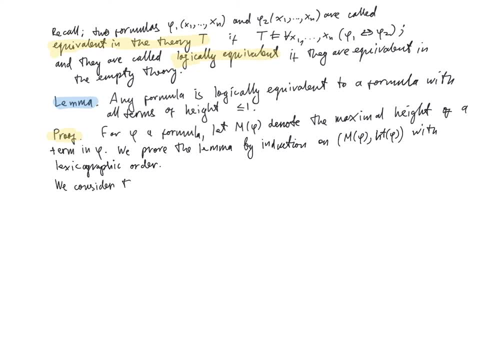 We consider the case when phi is an atomic formula of the form r, t1, tn. for some terms, this illustrates already the main idea, and the other cases are similar or even trivial. To simplify the notation, we assume that T1 is equal to T2.. 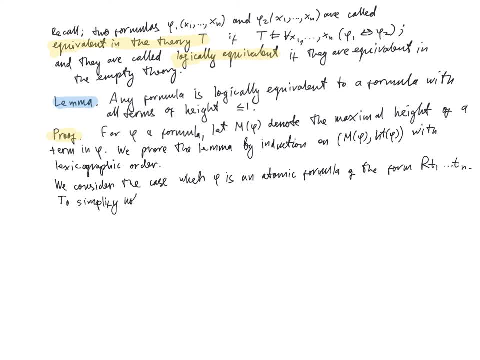 We put the values on the base of the formula. We plug in T1 and T2.. We interpret the equations as follows. We export them: that the height of each of the terms ti is greater than 1 for i ranging from 1 to m, and that the 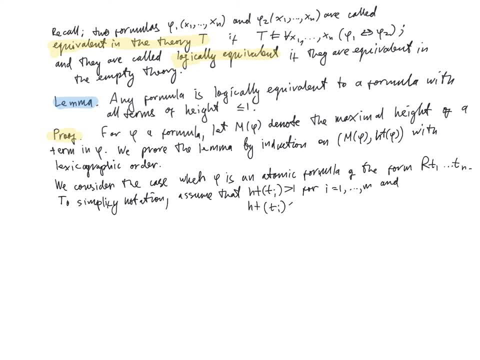 height of the terms ti is less or equal than 1 for i greater than m, So we might have to reorder the terms if necessary, but this does not lose any generality. For each i between 1 and m, let us write the term. 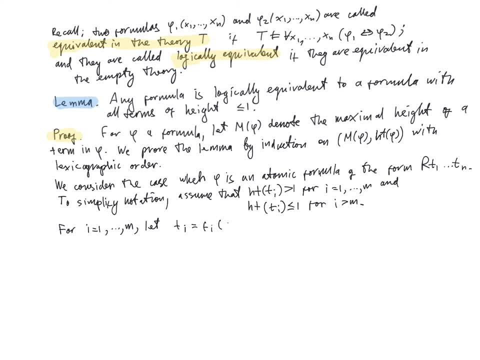 So we write the term ti sfi of si1 through siki. Since we assume that the height is greater than 1, it has to be of this term for some terms, si1 through siki. Then we choose new variables, yij for i, ranging over 1 through m and j between 1 and ki. Now if we write yi-bar to 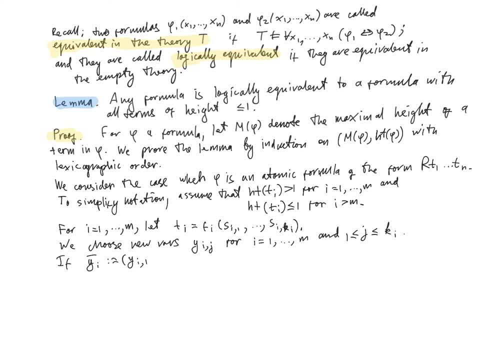 be the tuple of the variables yi1 through siki. So we write yi-bar to be the tuple of the variables yi1 through siki. Now, if we write yi-bar to be the tuple of the variables yi1 through siki, Then we choose new variables. yi-bar to be the tuple of the variables yi1 through siki. So we write yi-bar to be the tuple of the variables yi1 through siki, And we say that the height of the terms ti is less or equal to m For each i between 1 and m. let us write yi2 through siki. Then we 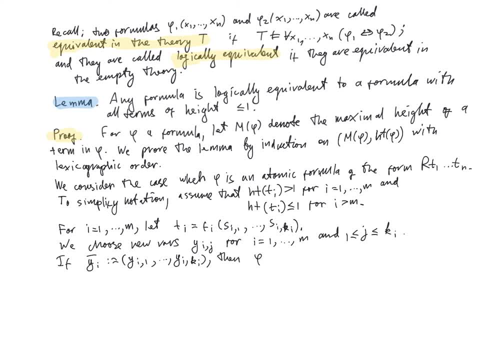 would add yi-bar to be the tuple of the variables yi1 through siki. Thus we have the strength value of the terms ti, and then we have the sum of them And here we have pi, with the result that is logically equivalent to the formula ψ given. 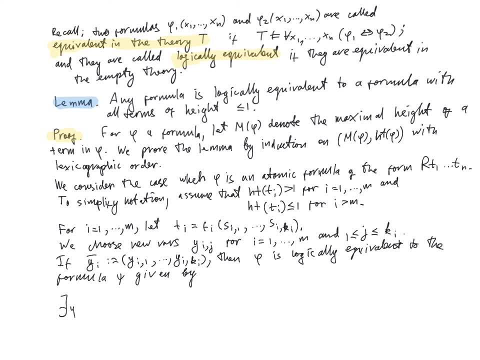 by the following expression: So we have exists Y1 bar through Ym bar, such that R F1 of Y1 bar through Fm of Ym bar, followed by the terms Tm plus 1 through Tn and conjunction overall Ij Yij is equal to Sij. 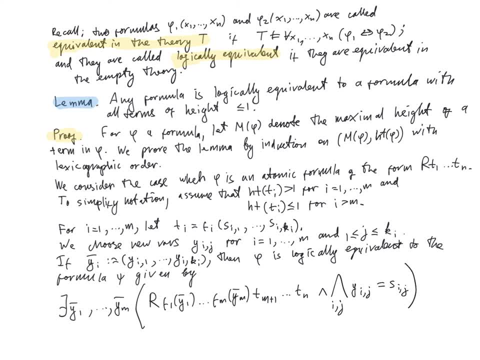 Note that the formula Psi written this way satisfies that M of Psi is strictly less than M of Psi. The case where the formula Psi is given by T1 is equal to T2, for some two terms is similar, So this shows that we can always reduce the maximal height of a term in a formula by 1. 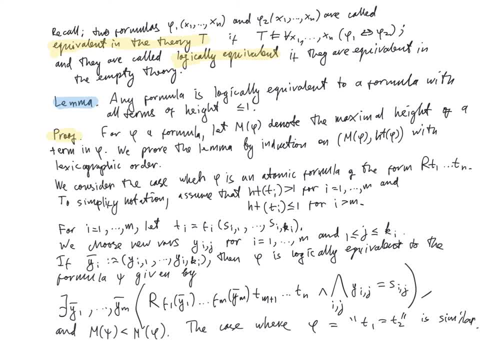 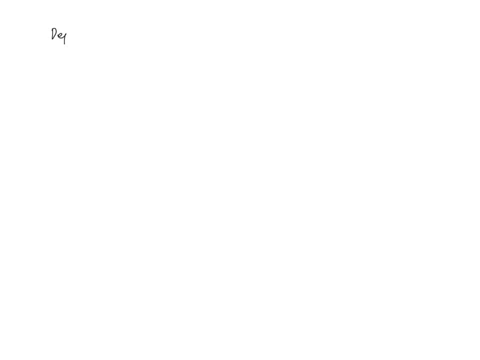 and repeating this, And this we will reduce to the situation with all terms of height 1.. Next, we have the following definition: Let T be an L-theory and assume that T' is a theory containing T in language L' Okay, For some, L' a language extending the language L. Then we say that T' is a conservative expansion. 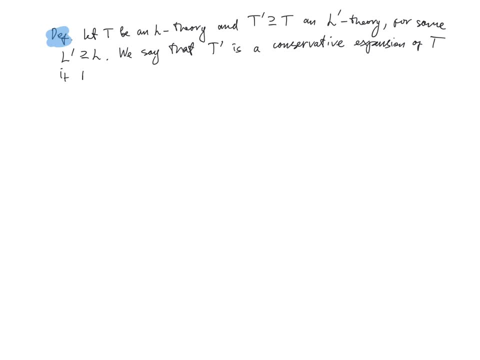 of T. Okay. Next we have the following definition: Let T be an L-theory and assume that T is a theory containing T in language L' Okay, For any L-sentence, Psi we have. T has Psi as a logical consequence if, and only if, 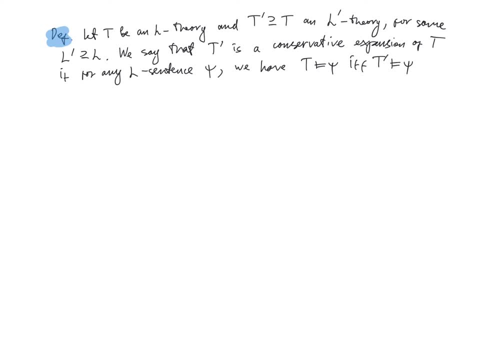 T' has Psi as a logical consequence. So even though T' is an expansion in a possibly larger language, At the level of the L-sentences it has exactly the same implications as T. And now we have the following proposition: Let T' be an expansion, by definition, of T. Then there is an expansion of T and we have: 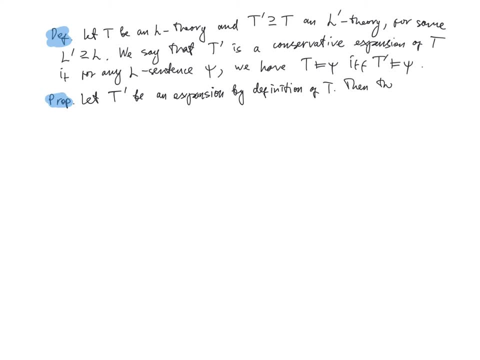 an expansion of T. Okay, So let's see a little bit more carefully. For example, if T' is a theory containing T, then the expansion T' of T is conservative. And furthermore we have that any L' formula Psi' is equivalent to a T' in language L'. 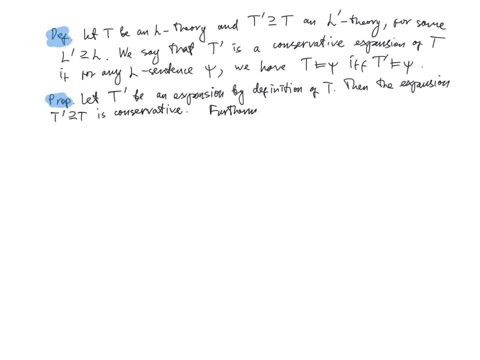 Okay, Now let's look at the next definition. Let T be an L' and assume that T is a theory containing T. Finally, let's see if T' is a theory containing T in language, Psi as a logical consequence. Okay, Let T be an L' and assume that T' has Psi as a logical consequence. 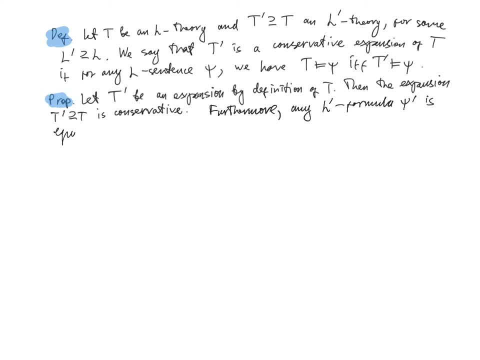 Okay, Let's look at the next definition: equivalent in T' to an L-formula Psi, Any model M of T has an L' expansion which is, in fact, unique to a model M' of T' Indeed, for a relation symbol R belonging to L' but not to L, we may define the interpretation. 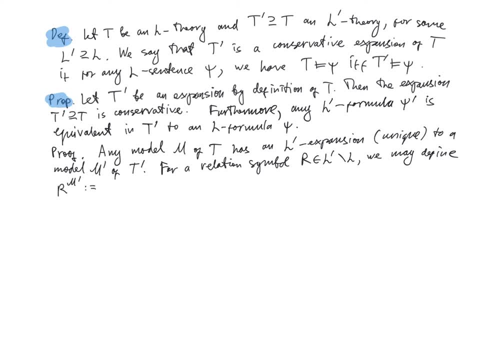 of R in M' to be the set of the realizations of the formula Psi R Given by the definitional expansion in the structure M, And it also follows from Beth's definability theorem, covered in the homework, that that's the only possible choice. 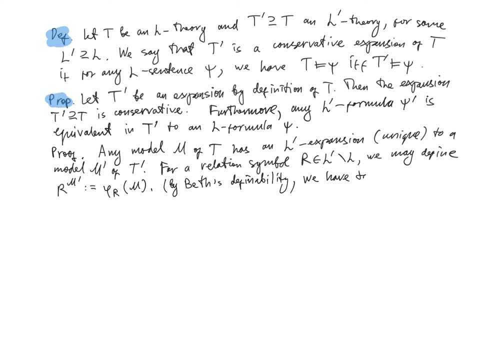 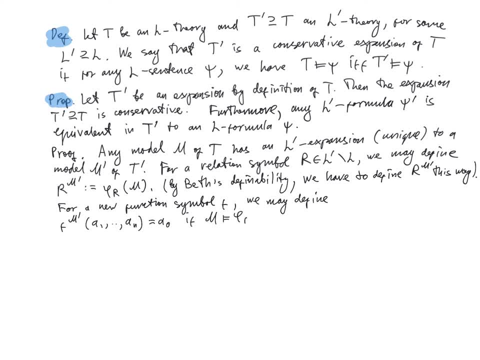 If we have that M satisfies the formula Phi F of a0, a1 through an And similarly, And similarly, And similarly for new constant symbols, We pick them to be the realizations of the corresponding formulas phi c, given in the definitional expansion. It then 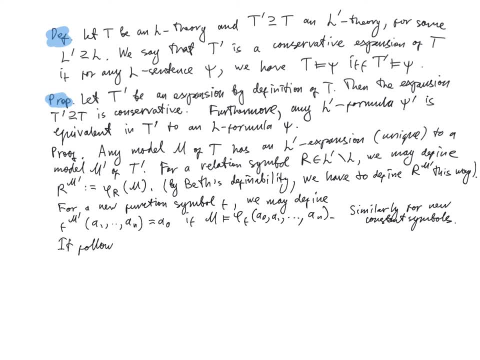 follows that T prime extending T is conservative, as any model of T can be expanded to a model of T prime. hence they have to have the same logical consequences. Now, in order to show that any L-prime formula is equivalent in the theory T prime to an L. 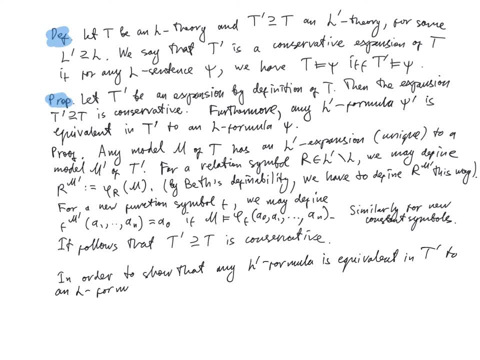 formula for simplicity, we will just treat the case where the expanded language L-prime consists of L together with a new function symbol for an anery function symbol, f. So we're just adding one single function symbol. The case of adding a relational symbol or a constant symbol are very similar, and the case of an art. 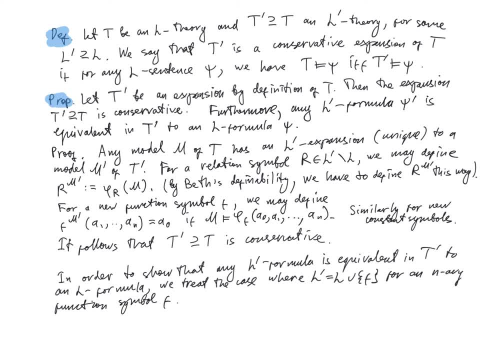 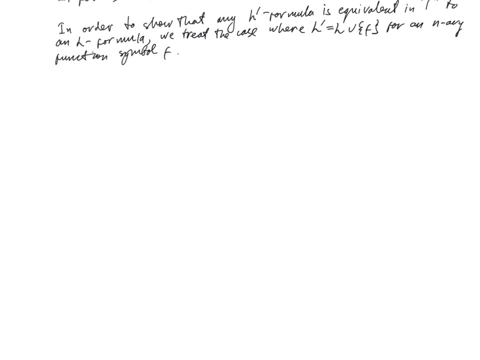 arbitrary expansion can be treated inductively by adding one symbol at a time of one of these three cases. So we'll just discuss the case of an anery function symbol. Let us first assume that xi, prime is an atomic formula, wieder 감. 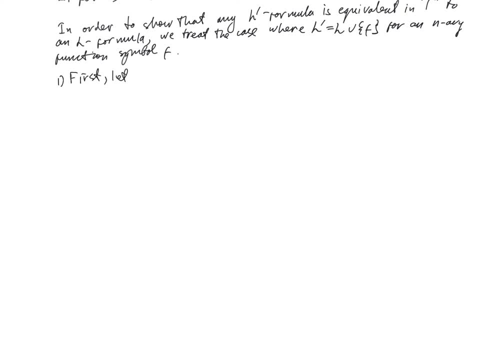 fomочно fom果 in the language L' containing only terms of height less or equal than 1, say, our formula of psi prime is of the form R, T1 through Tm. for some terms T1 through Tm. Assume also that for I, from 1 through K, we have that the term. 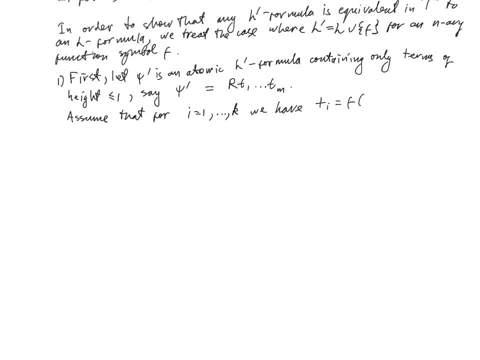 Ti is of the form F of S1i through SnI, for some terms S1i through SnI, And also that F does not appear in any of the terms Ti for I greater than 1.. This can always be achieved by rearranging the order of the terms, if needed. 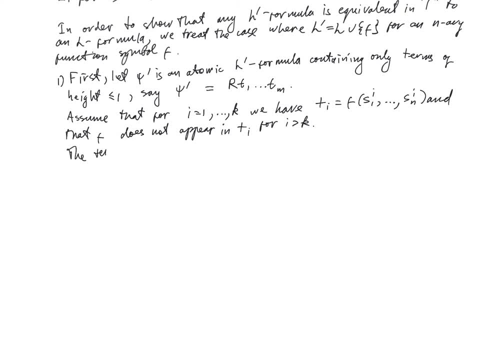 So then we have that the terms Sij all have height 0,, since we are assuming that all terms in psi prime have height at most 1.. So in particular Ti has height at most 1, thus they are all L terms, As we are assuming that F is the only new symbol in L prime that is not in L already. 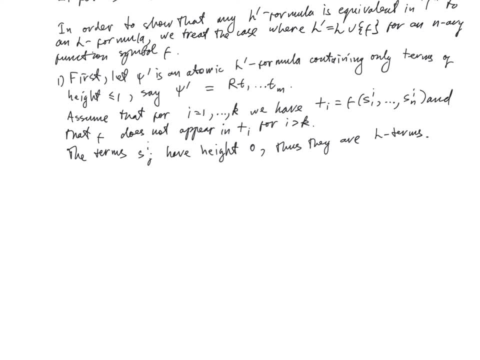 and each Sij has to be either a variable or a constant symbol. hence already in L. Now we let Z1 through ZK be new variables. Then the L formula given by Xist, Z1 through ZK, such that R Z1 through ZK is equal to: 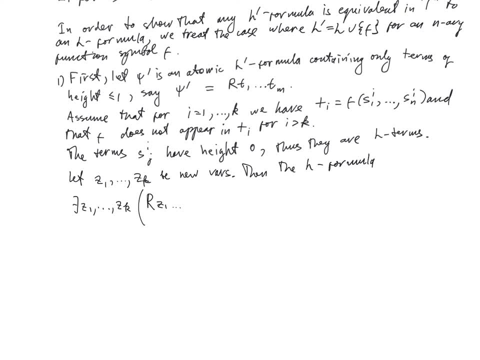 R, T1.. Each Sij has height 0. So we have same neurosis of these terms. Now we have to make our fermions z, k, t, k plus 1 through t, m and conjunction over i from 1 to k, phi of z, i, s1, i through. 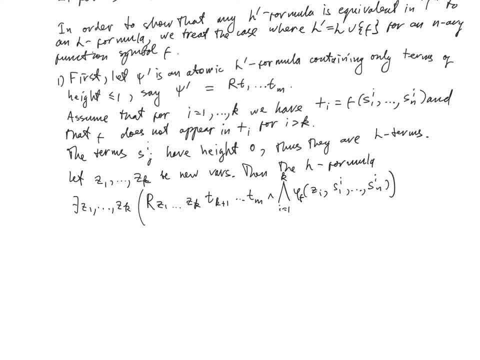 s n i is equivalent in t prime to the formula psi prime. That's because in a definitional expansion we know that the formula phi f, once we fix all of the variables except for the first one, We know that there exists a unique choice for the first variable. so the formula is satisfied. 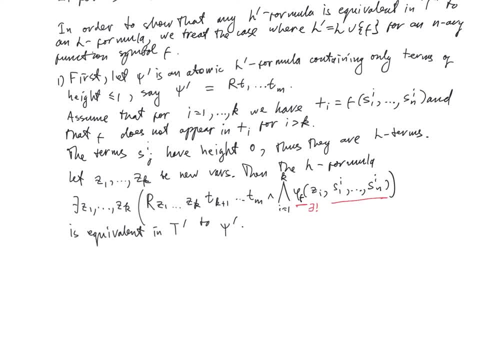 and we know that it is satisfied by applying f to the remaining variables 1 through n. So then we get that z1 through z, k represent exactly the results of applying f to the terms s1, i through s, n, i. because of this conjunction. 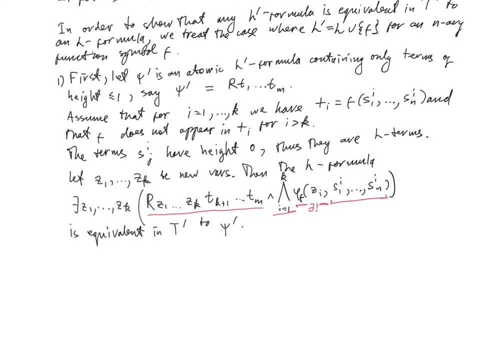 And then we express that r holds. So it is easy to see that we obtain a formula equivalent to the formula psi, prime, And this is indeed an L-formula, because r is a relational symbol, so hence must be already an L, because the only new symbol is the function symbol f. 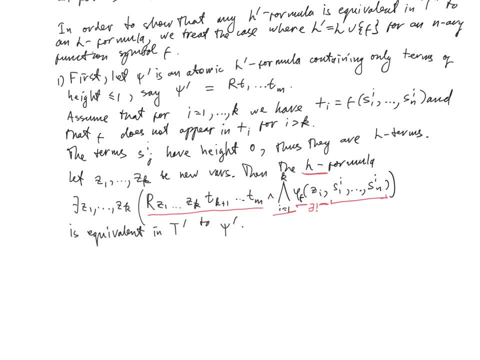 And phi f are of course, also L-formulas. Now, the other possibility is that psi prime is an L-formula. Now, the other possibility is that psi prime is an L-formula. Now, the other possibility is that psi prime is an L-formula. 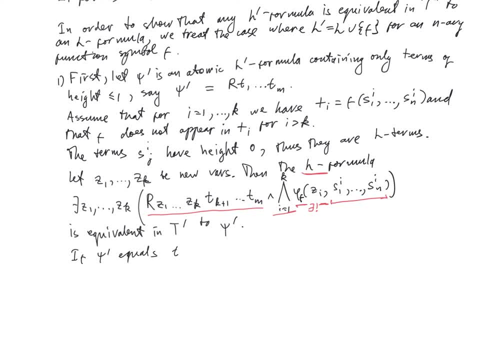 So when psi prime equals t1 equals t2- for some terms t1 and t2- then the argument is similar and we leave it out. So this deals with the case when psi prime is an L-formula which only contains terms of height less than or equal to 1.. 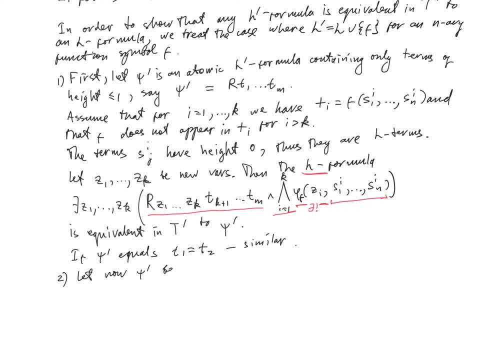 Now let psi prime. square root of psi n be is an atomic and sine squared. It is thus no point arguing phi it during. taking any example where the element p� quality in which it is homogn가지고 must have passes, be an arbitrary L' formula by the previous lemma. 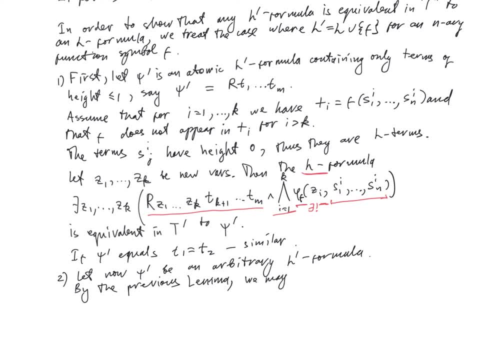 Up to logical equivalence, we may assume that all terms occurring in ψ' have height at most 1.. Now for any atomic subformula ψ' of ψ'. by part 1 of the proof there exists an L' formula chi equivalent. 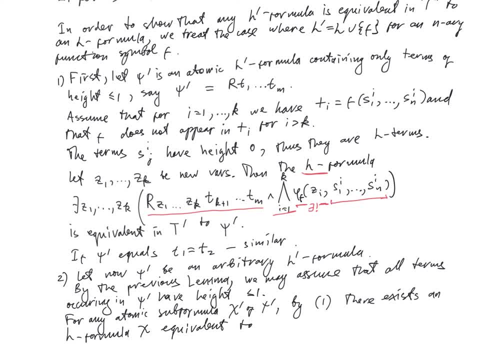 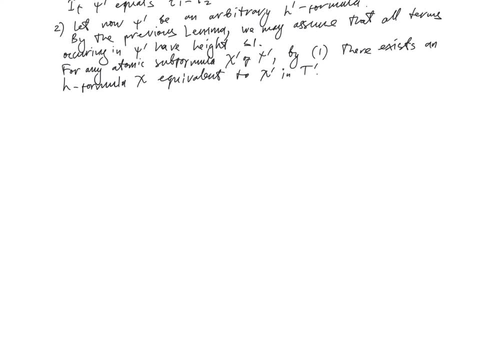 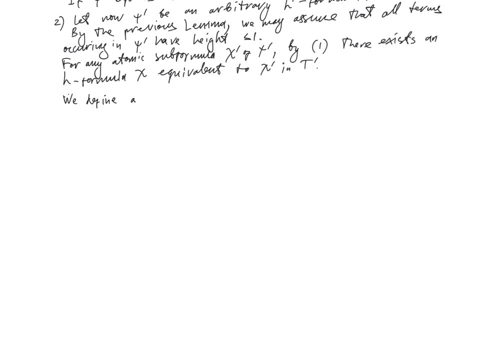 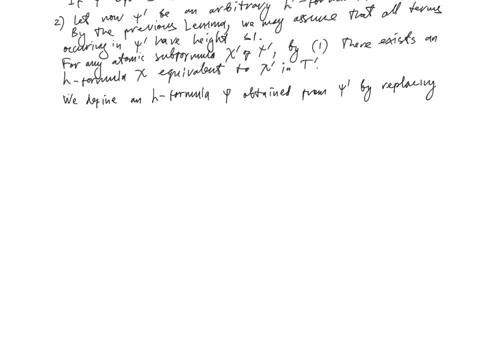 Of Christiv. it is an squares formula. every atomic subformula- chi prime of psi prime by an equivalent atomic L formula, chi. It remains to remark that we have the following general claim: replacing subformulas by equivalent ones produces an equivalent formula. We leave a proof of this claim as an exercise. 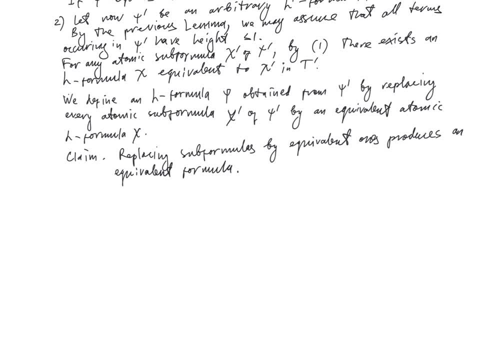 Let's consider a couple of examples of expansions. by definition. One: let T prime be the complete theory of the ordered field of real numbers. b tune strong. So it's a theory in the language L: Ordered rings. So it's a theory in the language L: Ordered rings. 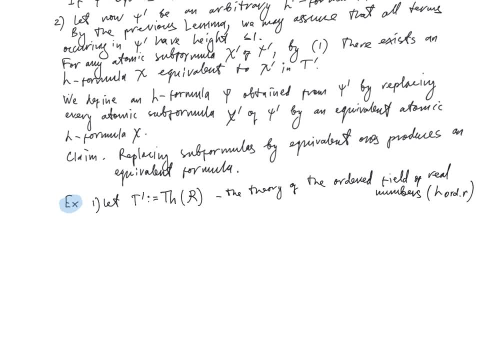 So it's a theory. in the language L Ordered rings An. we also let n be Forgive if kommt to a real number. S is non- cellular. we also let T be the theory of the field of real numbers. so the field of real numbers. 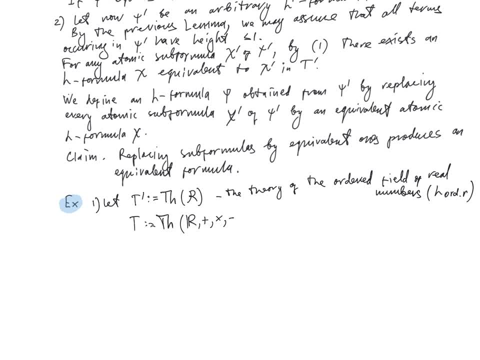 with the operation of addition, multiplication and subtraction and constant 0, 1.. So this is the theory of the field of real numbers in the language of rings, so a smaller language. but now we have that in R. we have that R is less than S for two real numbers, if, and only if, there exists. 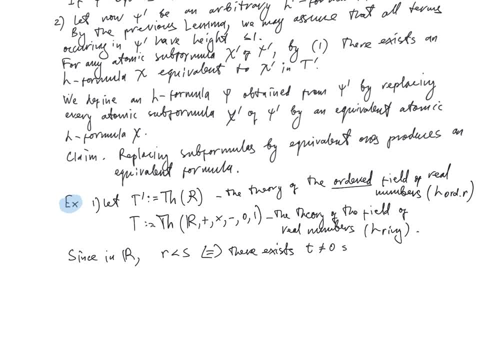 a real number T different from zero, such that T square is equal to S minus R. it follows that T prime is an expansion by definition of T, as this condition can be expressed by a formula, and hence we can write a formula phi less than in two free variables, x and y. 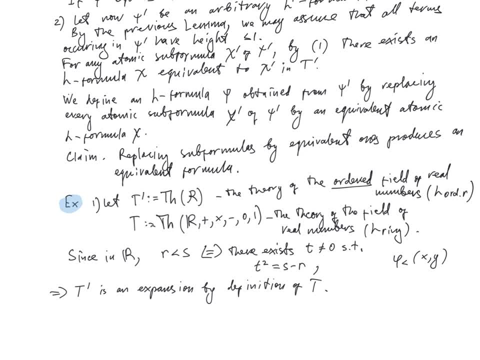 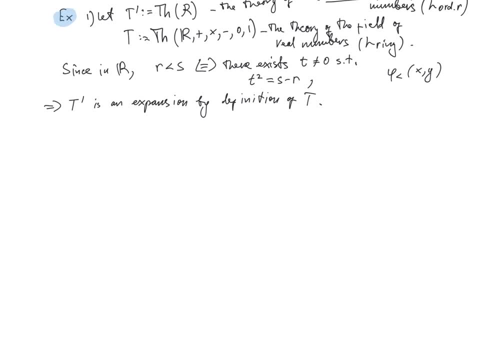 which is going to hold precisely when x is less than y. Example 2,. let's see the theory in the language of linear orders. let this be the theory of total orders without endpoints. note that this can be expressed by a sentence saying that for each element, there exists an. 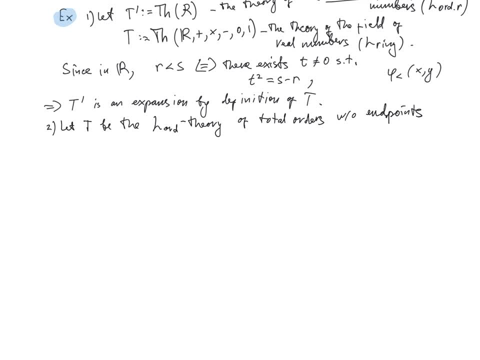 element greater than it and for every x there exists y less than it, and we also let T prime be the theory in the language of ordered rings, which is the theory of ordered fields. so the axiom for fields and axiom expressing that the order is compatible with the field operations. 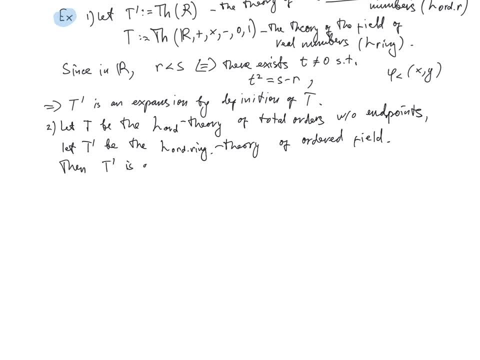 then we have that T prime is a non-conservative expansion of T. so we have that T prime implies that for all x, for all y, x less than y implies there exists z, x is less than z and z is less than y. 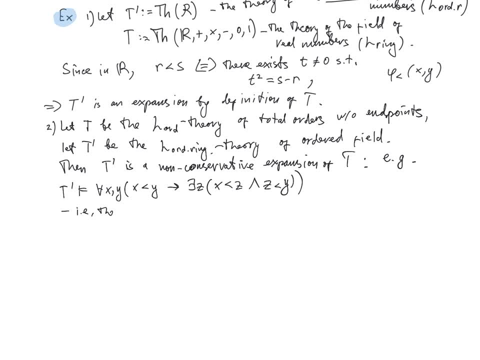 in other words, the order in any ordered field is dense, and the reason for this is that, given any pair of points, we can look at the interval that they define and then it has a midpoint, which can be expressed as x plus y over 2,. 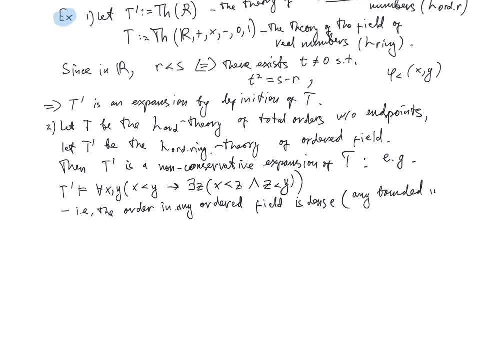 so any bounded interval has a midpoint which is expressible by the field's operations. hence the order has to be dense. but this density is not a logical consequence of T sounds cool because of course we can have linear orders without end-points which are not dense. 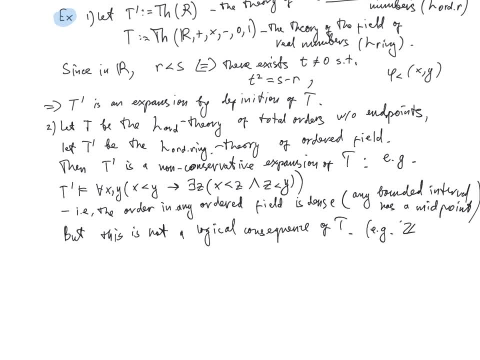 so, for example, z with the linear ordering satisfies T, shows that there's an else sentence which is a consequence of T prime but not of T. hence this is not a conservative expansion. Example 3, let T be the theory of the ordinal omega 1, together with the 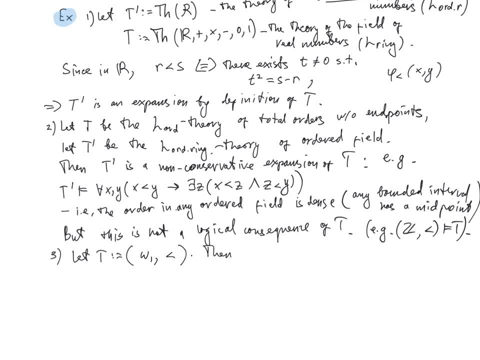 linear ordering on it. So this is an L-ord theory. Then we have that the element omega is a definable constant in T, meaning that there exists a formula phi of x0, such that T implies exists a unique formula. So this is an L-ord theory. Then we have that the element omega is a definable constant in T, meaning that there exists a formula phi of x0, such that T implies exists a unique. 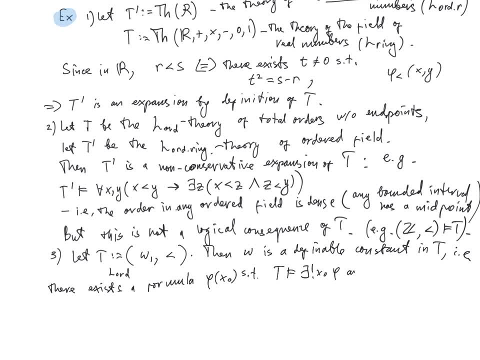 x0, such that phi, And so that omega 1, with the order, satisfies phi of omega, which is of course an element of omega 1.. So, indeed, the set of limit ordinals is defined by the formula lim of x, which says: exists y, y is less than x and for: